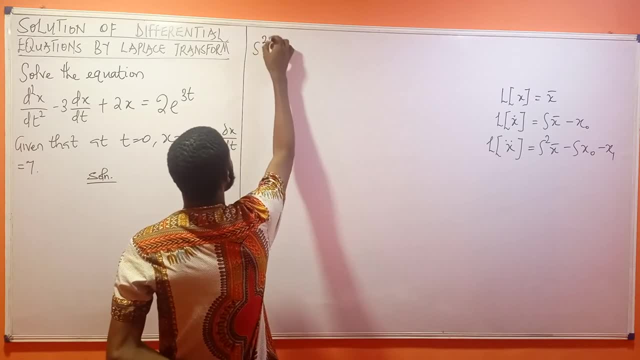 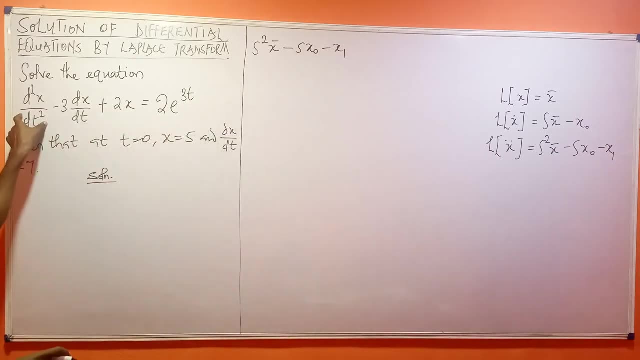 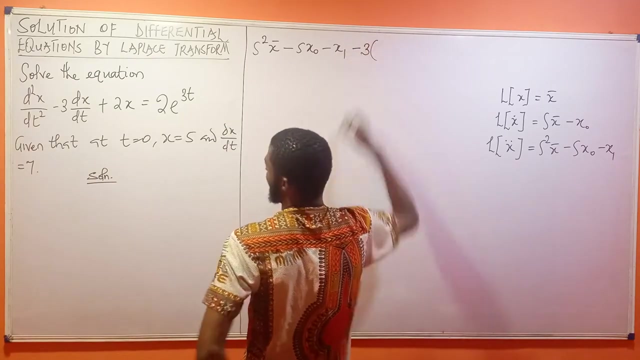 what is it going to give to us? It is what s squared s bar minus s s naught minus x one. So that's for the what. This is second derivative. When you take the Laplace transform, that's what you are going to get here. So this is minus three brackets If you take the Laplace transform of the. 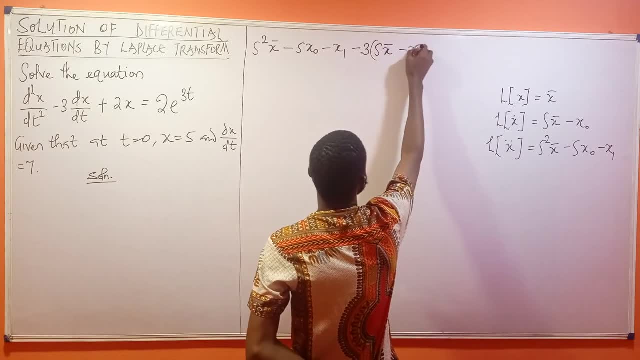 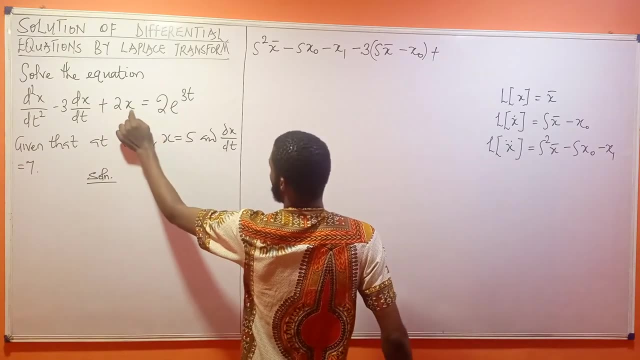 derivative. this is it. You're going to have s s bar minus s naught. Then close the bracket, Then plus two. If you take the Laplace transform of s, s is going to give you what s bar. So this is two. 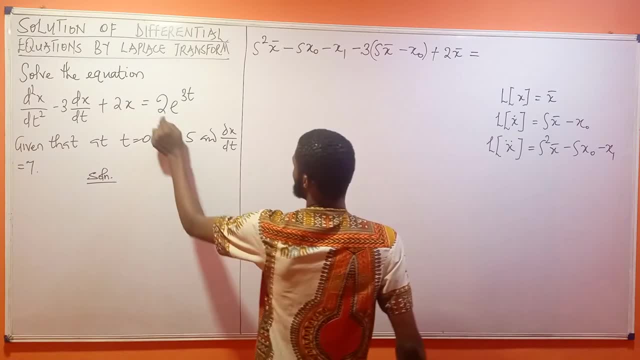 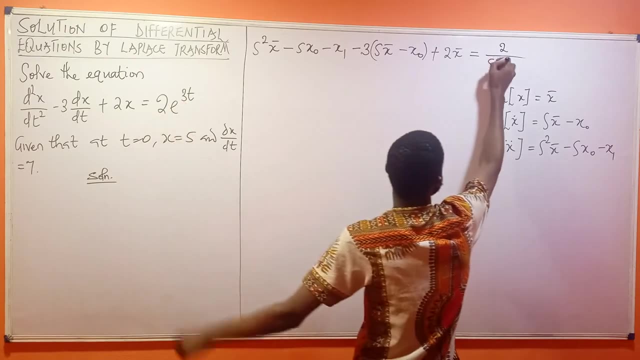 s bar, Then equal Laplace transform of two e. So first of all, you have two over. as a result of this three here we're going to have s minus three. Remember, I said you need to start from the first video so that you get hold of this. So you're going to have s minus three. So you're going to 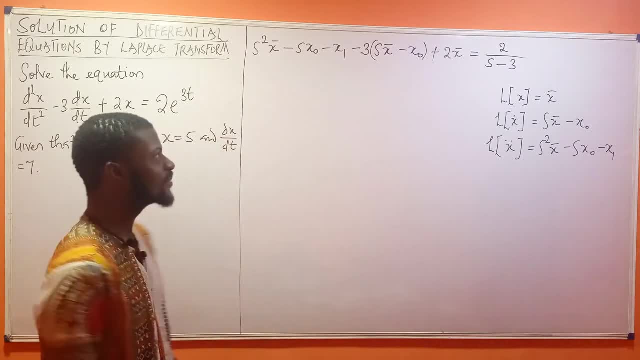 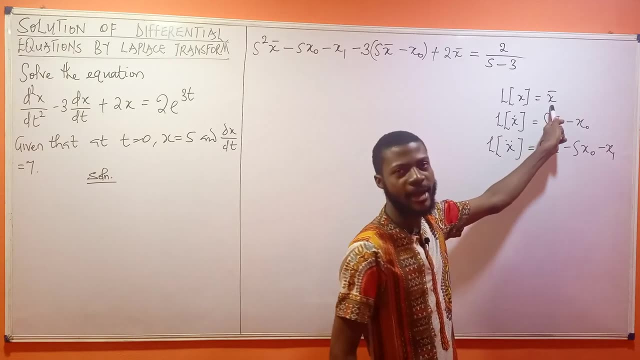 get hold of this properly. Wow, this is actually long, but it's easy. It's very, very easy. Now, what is the main thing we're trying to do here? We're trying to solve for what s bar, So we're going to. 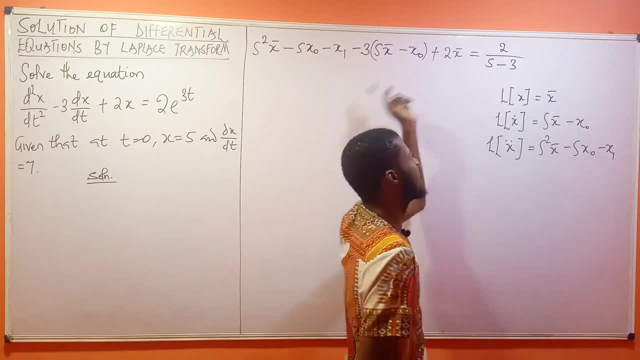 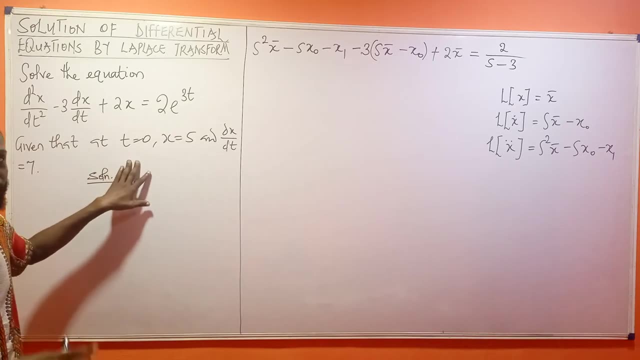 make s bar. So we're going to express everything in terms of s bar. So let us get started with that. But before we do that, what is the initial condition I was giving to you? After writing everything in terms of their transform, the next thing is to put in the parameters, So write a. 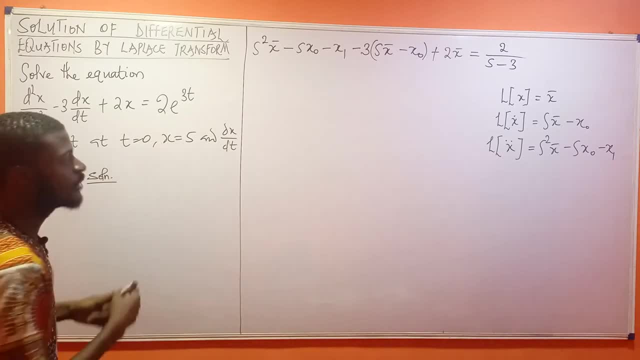 little bit about the initial condition. s is equal to five, Please take note. this means s naught is equal to five. Then ds dt means x1.. I think I've explained this in my first video. So s naught is equal to five, Then ds dt will become x1. and this is what Seven. What if you were giving d squared? 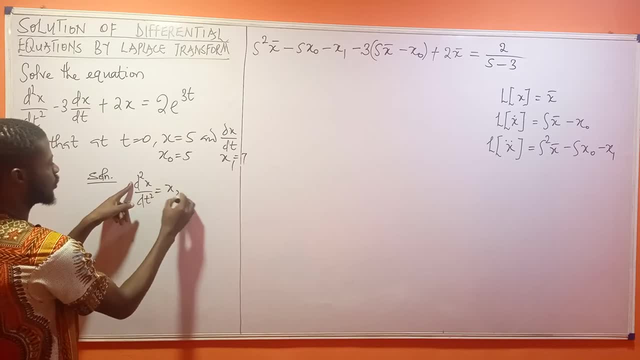 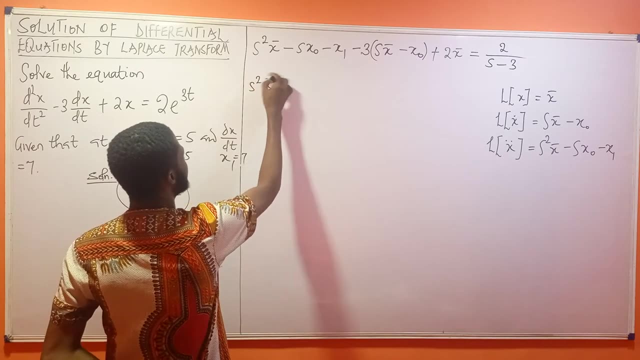 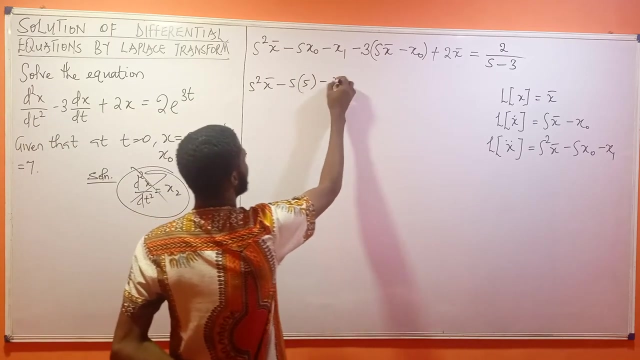 s over dt squared. This thing means what s2.. But we're not using that in this very question, So let us take a look at what we're going to do here. So we're going to write s bar minus s bracket: What? 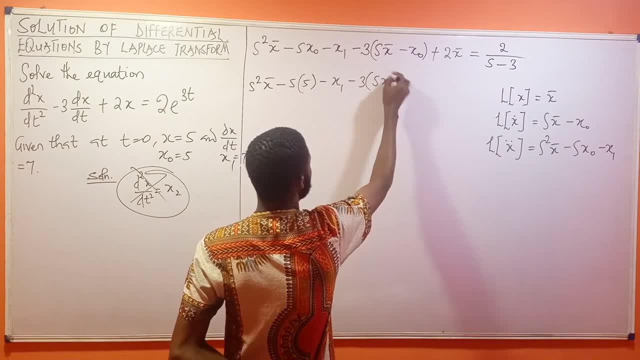 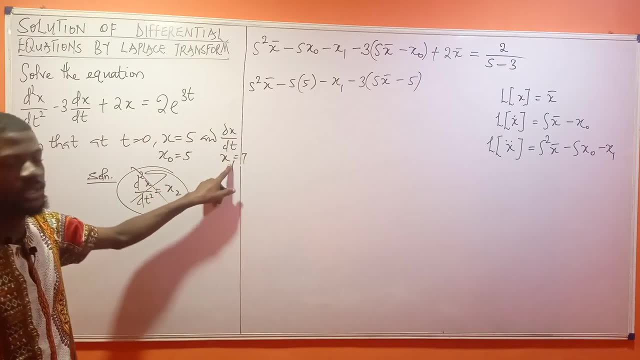 is s naught. s naught is five. Then minus s1, minus three, bracket s s bar minus five. Remember that s naught is what Five. Now, what is s1?? s1 is equal to what Seven, So I can just remove this s1 and 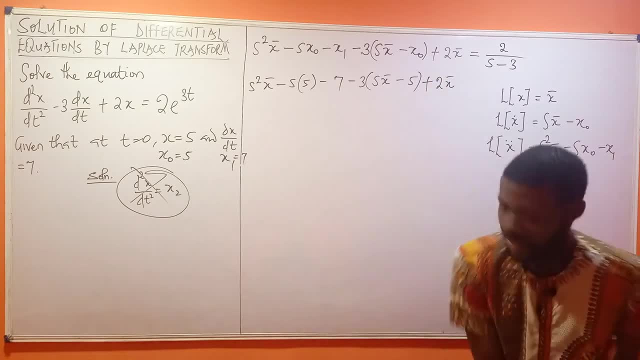 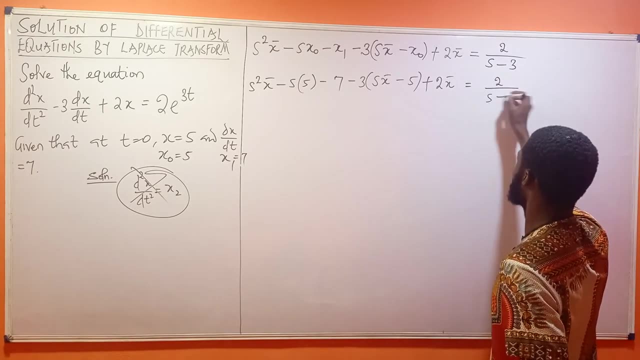 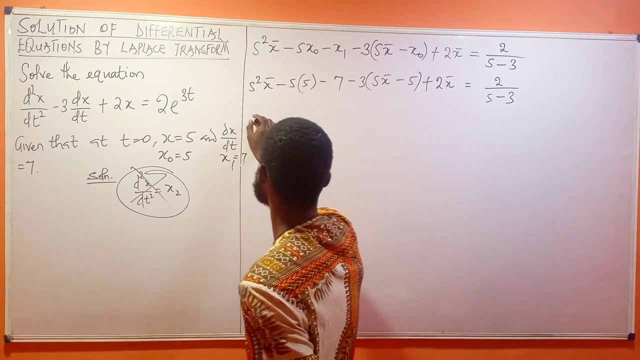 write seven, I think I did say that earlier. Then plus two s bar. Then obviously this other side is going to wipe it off. Then a equal to two over s minus three. Okay, let us proceed Now. let me open the brackets. So this is s squared s bar minus five times. s will give us five s, Then minus seven. 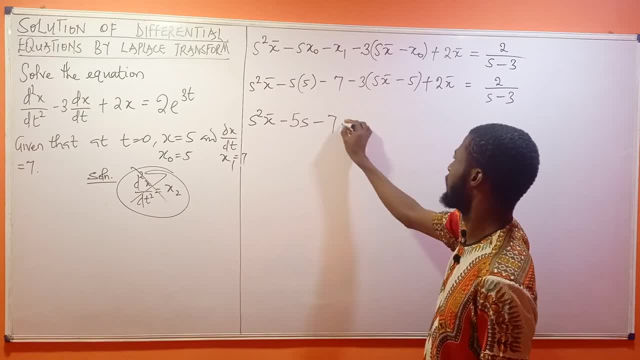 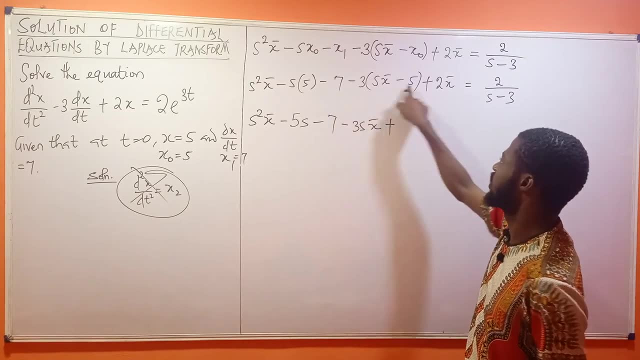 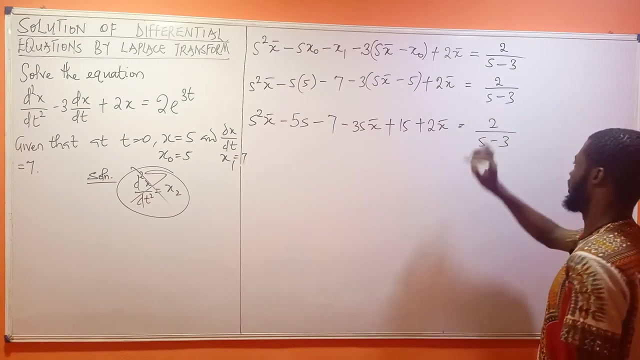 minus three s times. this will give me minus three s s bar. So that's what I'm going to be having: The minus times minus here will give me plus Five, fifteen, Then plus two x bar equal two over s minus three. So this is what we're going to be. 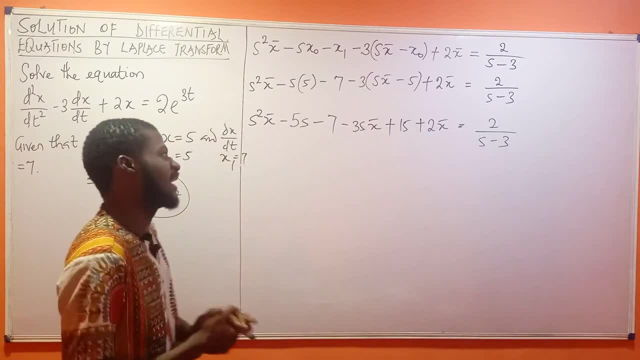 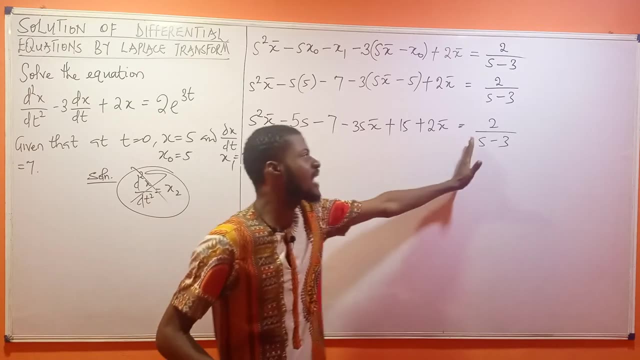 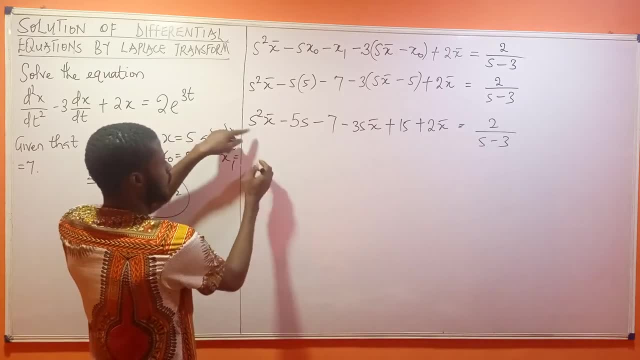 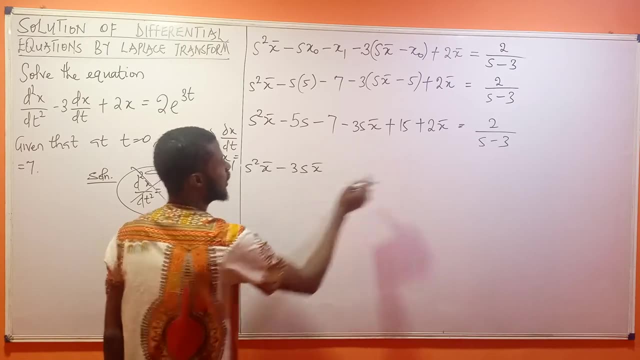 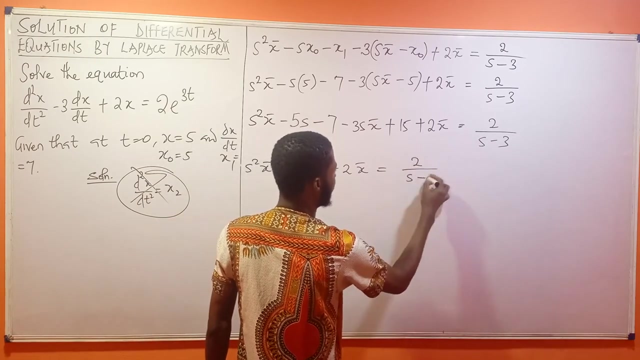 more convenient that way. So this s squared, this s squared s bar. It's going to remain This guy minus three s s bar is going to remain. Then plus two s bar is going to remain Equal to. on this other side, we'll have two over s minus three If minus five s goes away. 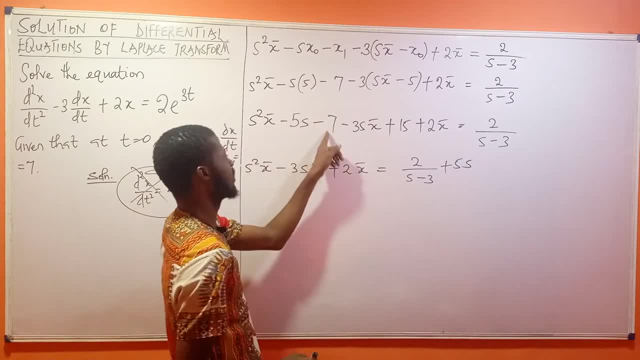 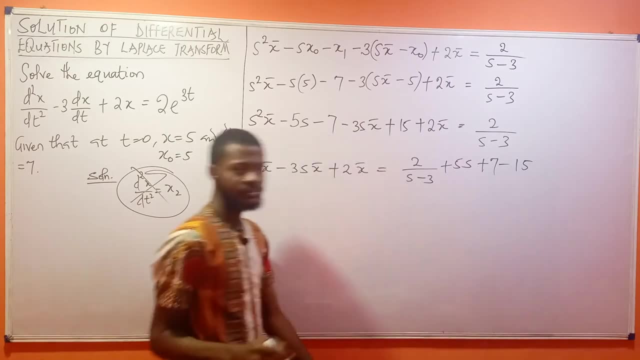 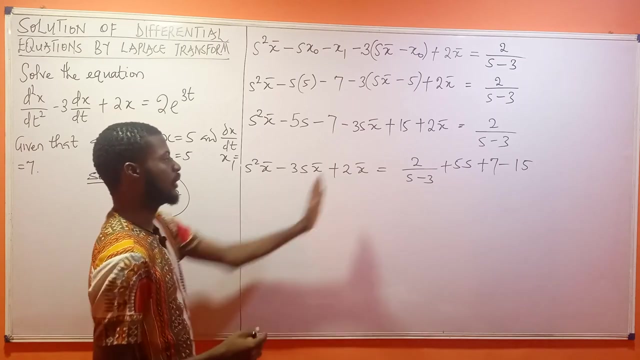 to become what Plus five s. If minus seven goes away, to become what Plus seven. If fifteen goes away, to become what Minus fifteen. So that's correct. So let us proceed Now. looking at this expression that you're seeing, This expression that you're seeing What's totally common with 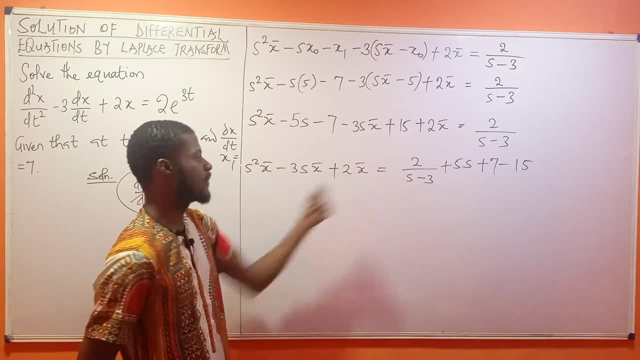 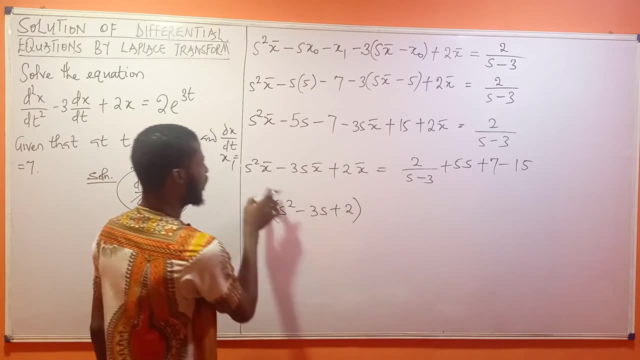 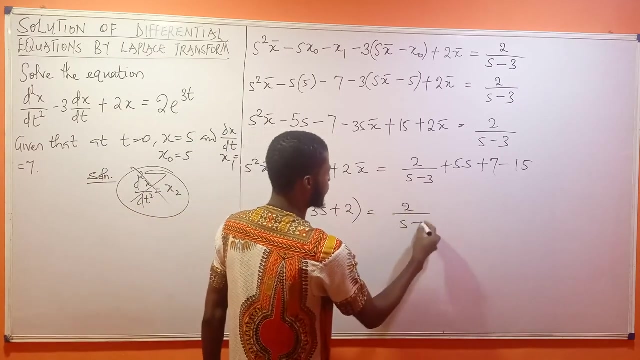 this side. You can see s bar is here, x bar is here, x bar is here. So this is x bar bracket s squared minus three s plus two. If you factorize s bar out of this expression, you're going to be having this remaining Equal to two over s minus three plus five. x Seven minus five should be. 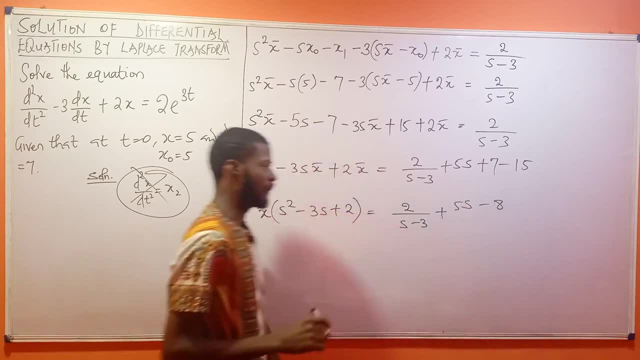 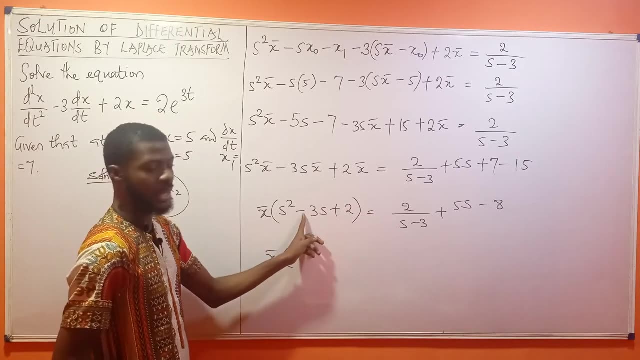 eight, So this is minus eight. Okay, So this is what we have. Now, this is what we have. This is x bar bracket. Is this factorizable? Yes, it is. This is minus three and this is two, So it's. 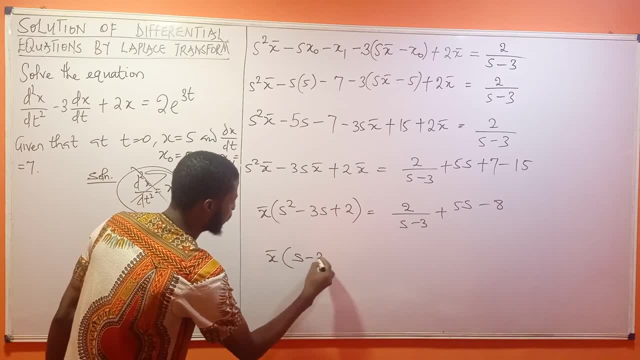 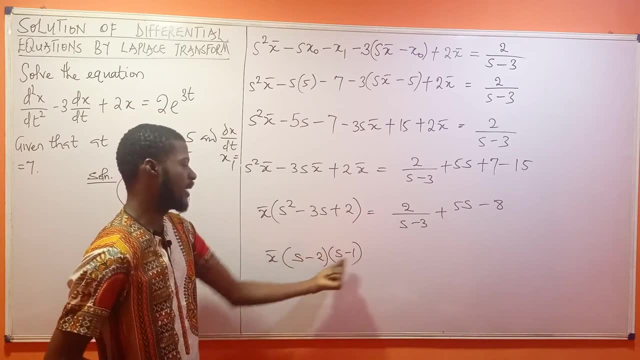 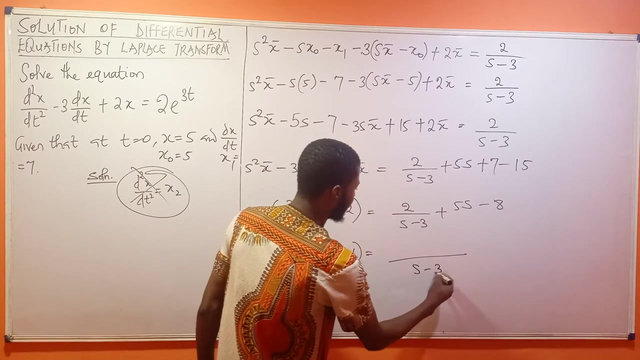 factorizable. So what about now? What would this give to us? S minus two. brackets s minus one. Yes, because the numbers you can times to get to and only to get minus three, The numbers are minus one and minus two Equal to um. okay, This very side, the lcm here, is s minus three. I'm going to be 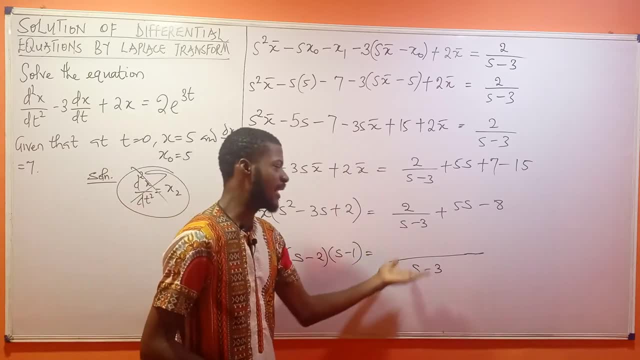 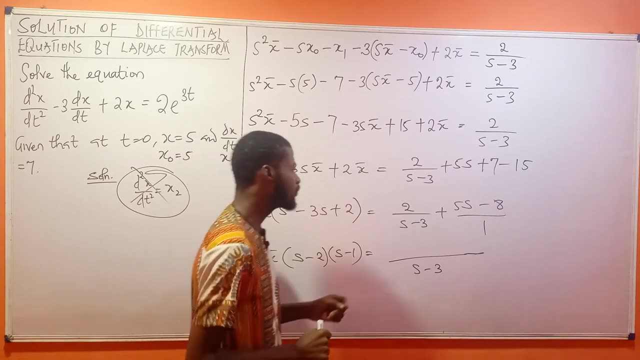 doing this very fast. So we're asked to actually expand. like you know, We're going to do fc. I'm going to say um over one here, But maybe we do not have that time. So what I'm going to do Five s times, this s here is going to give me five s squared. So this is five. 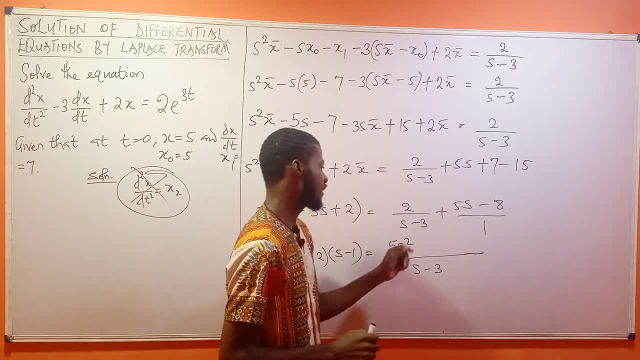 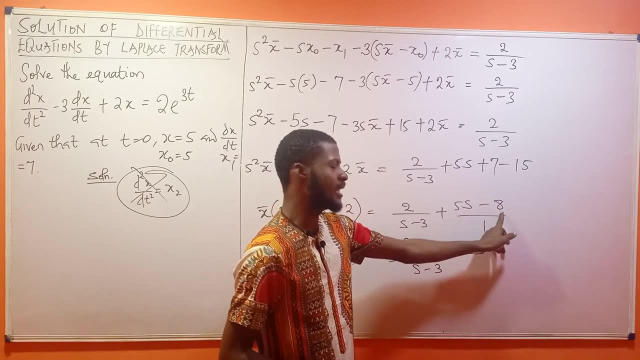 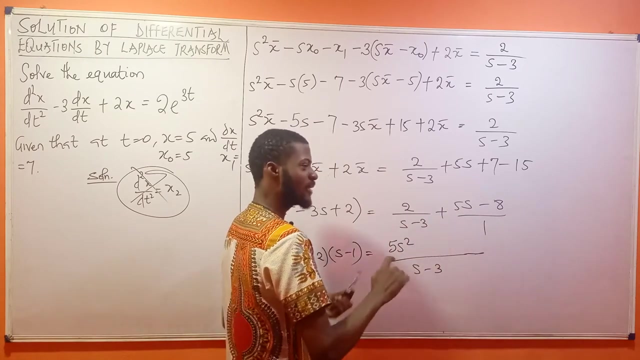 s squared, Then the next I'm going to do is um the s guy. I'm going to say um, where is it s times? minus eight will give me minus eight. Now, minus three times five s is going to give me minus fifteen s Minus eight minus five is going to give me minus fifteen s Minus three times five s is. 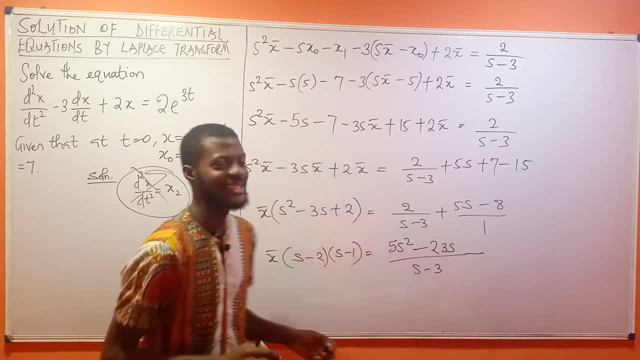 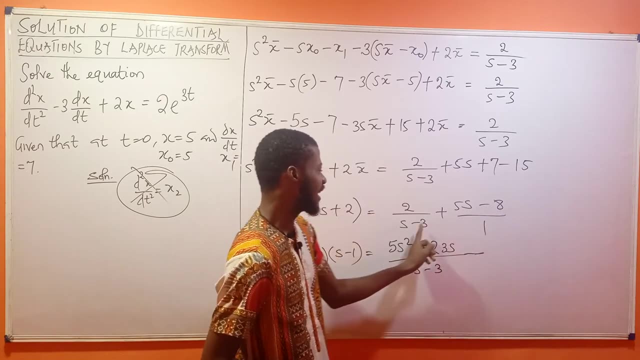 going to give me minus fifteen will give you minus twenty three s. Actually, there's a way I do all of these things very, very fast, But the answer is correct. Then this other one, minus eight times minus three, will give us twenty four. Twenty four plus this very two will become twenty six. Yeah, 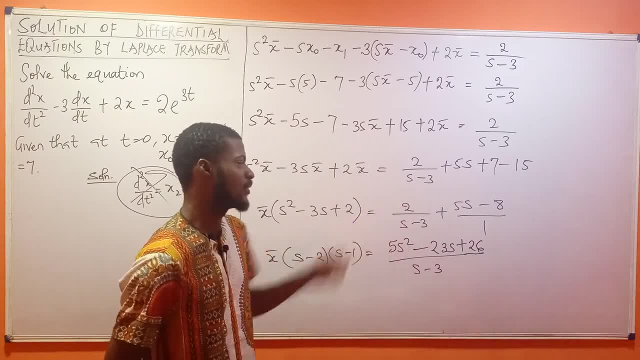 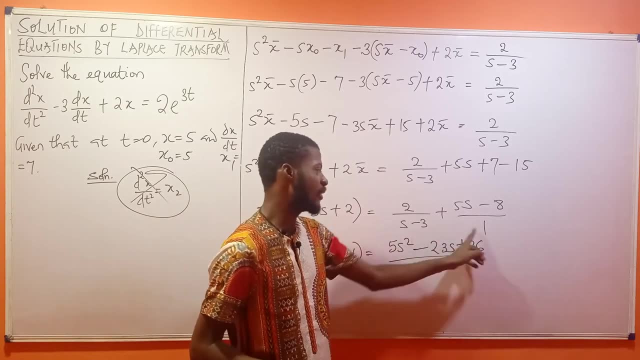 it's obvious. this two is going to be useful when we have constants. So this is what I'm going to get Now. if you do not understand this, you can actually- you know- rule a line, Then take the lcm of both sides. When you take the lcm of both sides, you're going to still have the same expression. 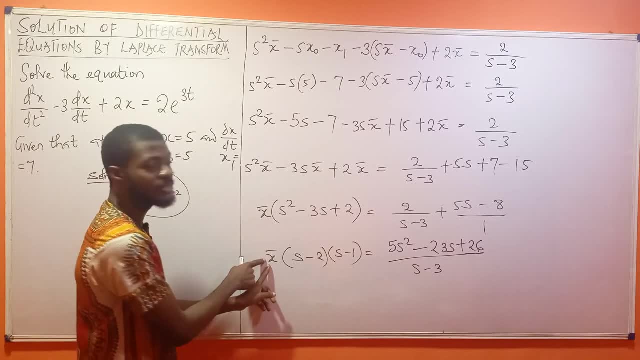 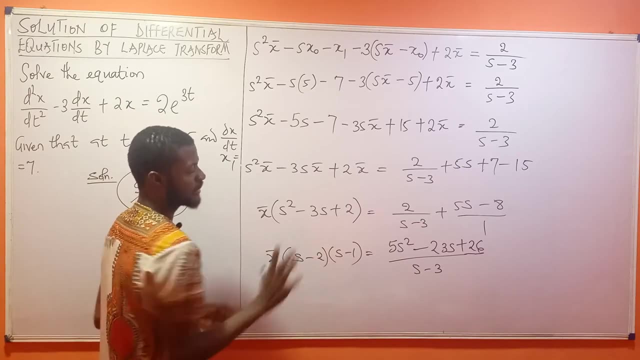 You're going to end up there, But the next I'm going to do is this: I'm concerned with making this very expression have only s bar at this very side. So what do I need to do? Divide both sides by what s minus two s minus one. So when I do that, I'm going to have s bar equal um five s squared. 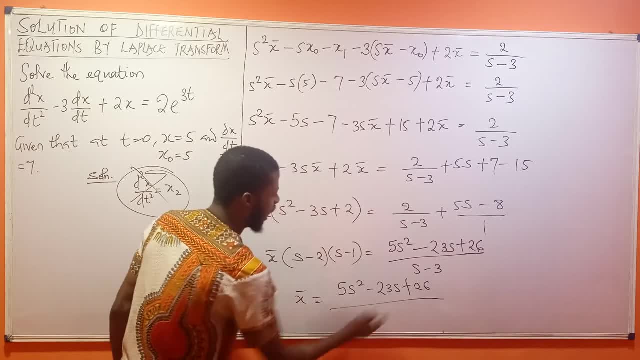 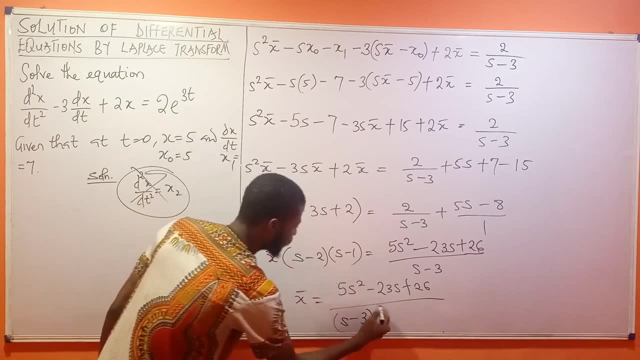 minus twenty three. s plus twenty six, divided by the first denominator here is s minus three. Then I'm going to be divided by this two. So it's obvious these two guys will be coming under. So this is s minus two bracket s minus one. 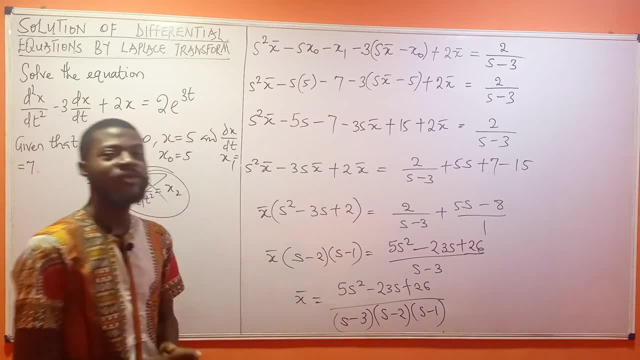 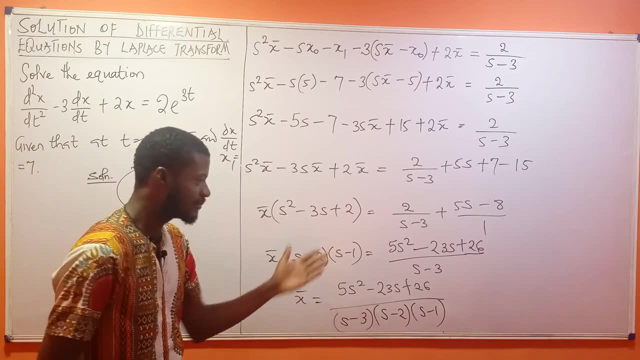 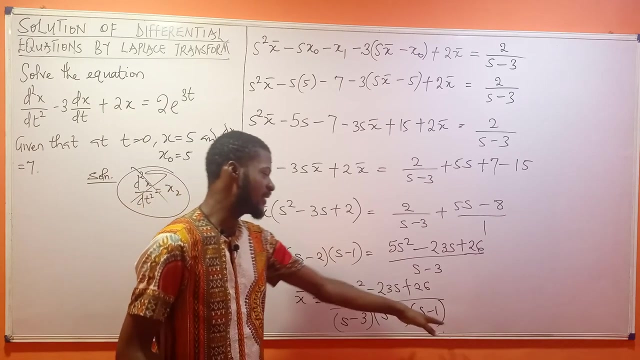 Beautiful. So this is what we'll have Now for this very expression. we are concerned with finding a, b, c. and what Nothing? a, b and c. because we have just three factors at the denominator and they are linear factors, So it's just a, b, c. Now we're going to be doing it very fast, Very, very. 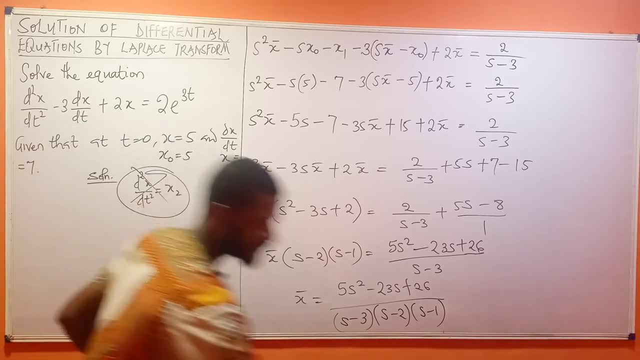 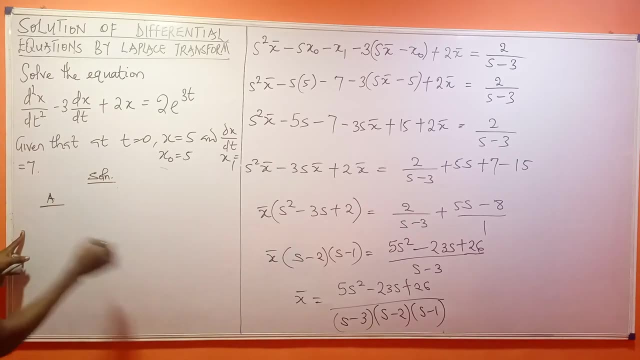 fast. Okay, let me, I think I'm going, I can be able to do it here, I'm able to do it on this very side. So let us say the expression is equal to a over first denominator. there is s minus three plus b over second denominator, s minus two plus. 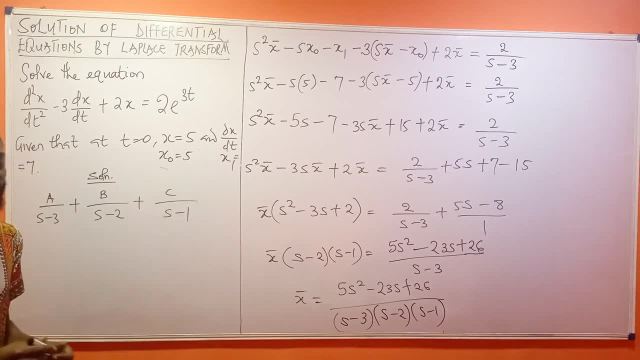 c over last denominator s minus one. So let me- let's just do that very, very fast. Now see what I'm going to do. I'm going to be using cover up because it's very easy for me to do, So let me get. 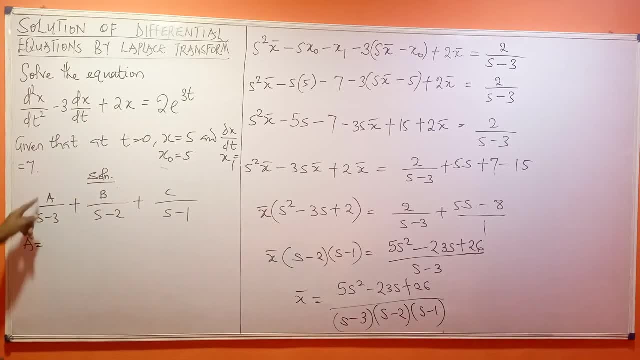 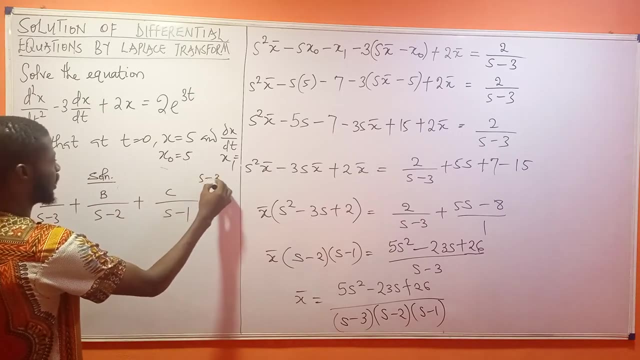 my a. If I'm going to be starting with a, what's at the denominator of a, s minus three. So I'm going to say s minus three should be equal to zero. So if you say s minus three equal to zero, your s will become what Three, Because minus three will go to what The. 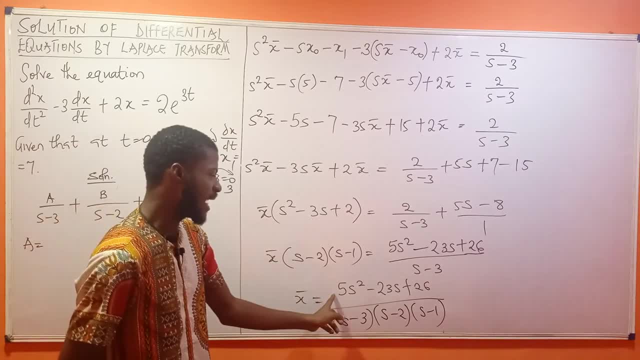 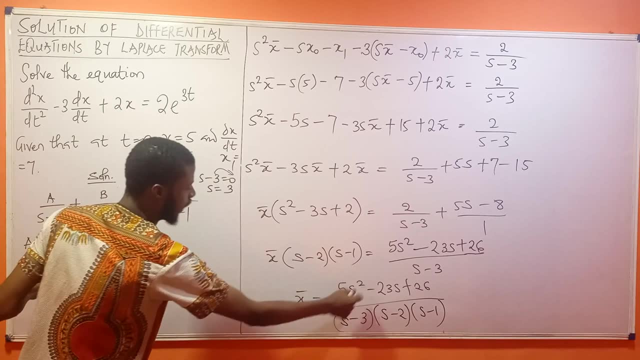 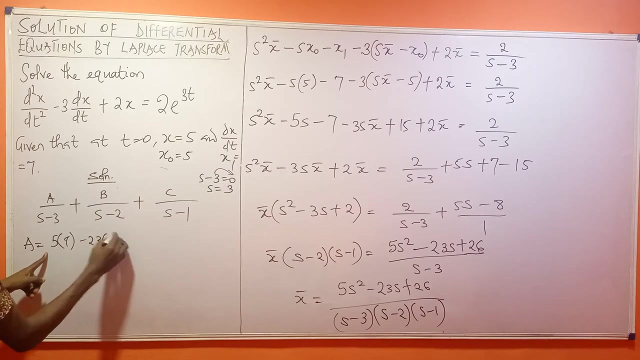 other side. So you then have three. So, anyway, you see s at this very fraction, So I'm going to put what Three. So let us get started. This is five brackets s squared. Three squared is what Nine. So this is brackets nine minus 23. brackets three plus 26. divided by this is s minus three, Remember. 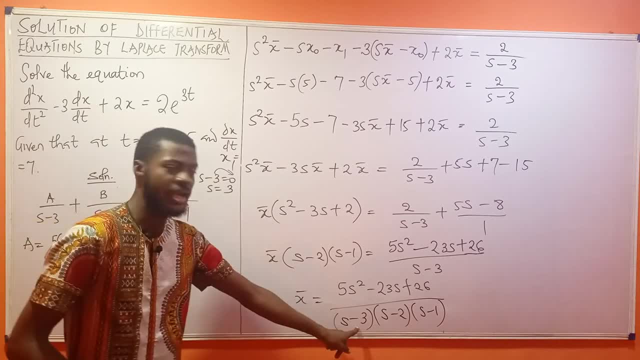 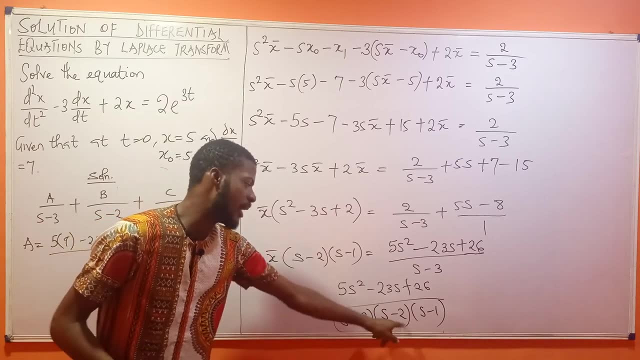 I used s minus three to get my value of s. I'm not going to put it here because I'm going to be having zero to just spoil the whole expression and it becomes undefined. So we can't be doing that. So go to s minus two. When you say three minus two, what are you going to have? You're going to have: 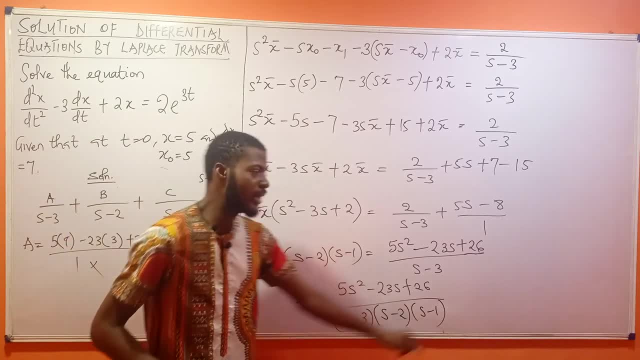 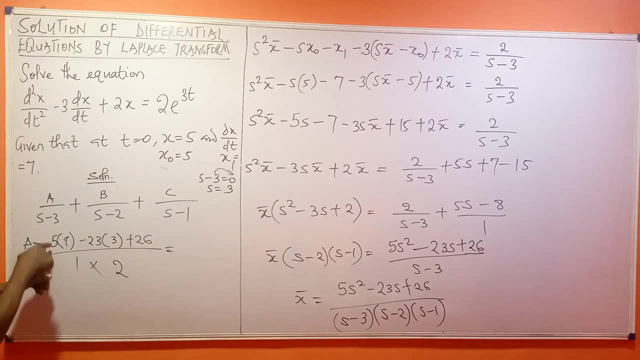 one times. When you say three minus one, what are you going to be having? Two, Remember anyway, you see s you are putting what Three. So right now, what is this expression going to be at the end of the day? Five times this will give us forty. five minus twenty. three times three will give us sixty. 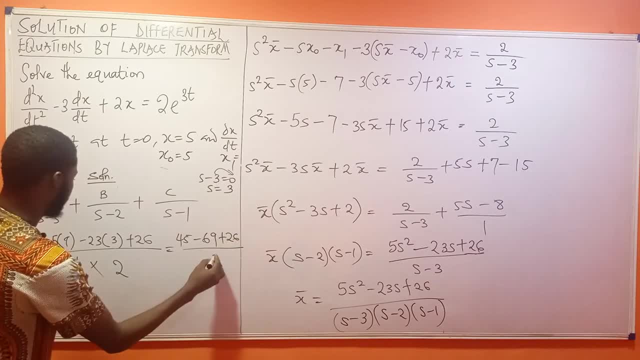 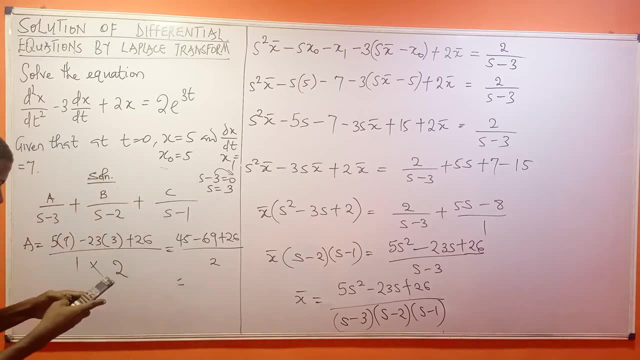 nine, Then plus what Twenty six, Divided by what, Two. So what's your a? finally, A is going to become forty five minus this, so sixty nine. Okay, so a is one. So when you divide that by two, you're going to get one. So that's divided. 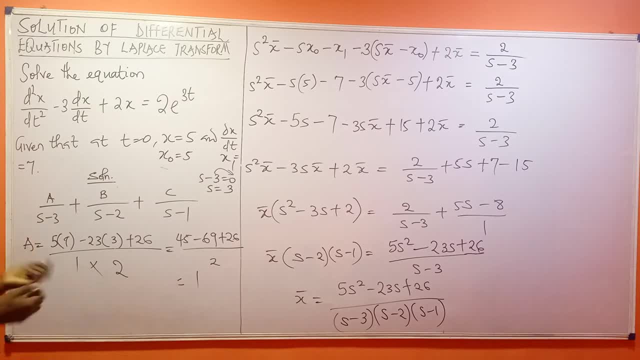 for a. So we've gotten our a very, very fast. Then b: What will b become at the end of the day? Below b we have x minus two. So how do I get my answer for b? I can wipe this part of the board. 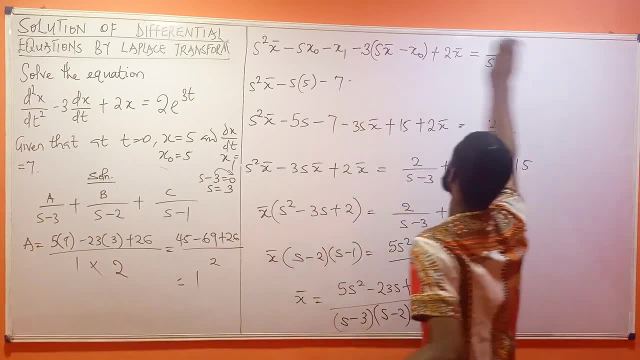 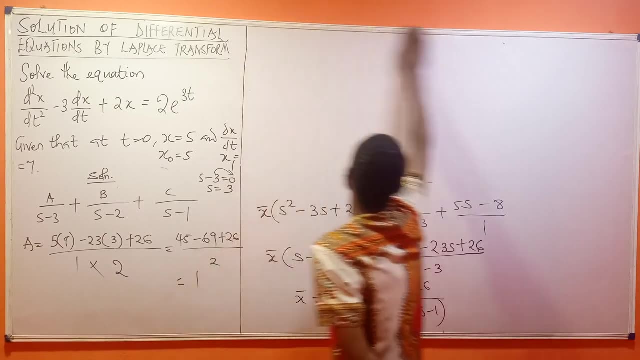 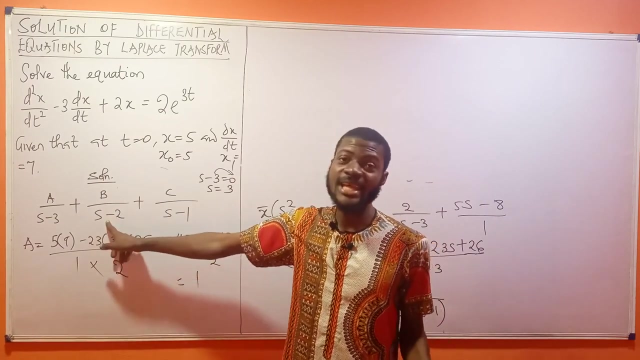 now I think you've taken a screenshot already. So to get our b, Okay, so to get b at the bottom of b, I have s minus two. So what does this mean? S has to become two. That's the meaning S has to. 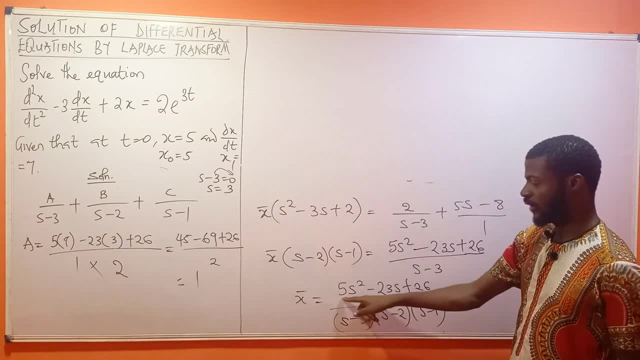 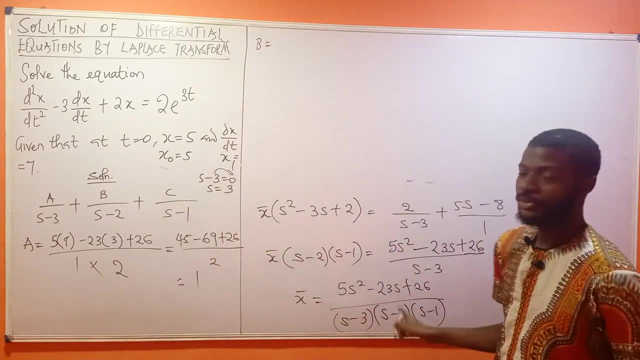 become what Two. So this is the expression that I have here. So, anyway, I see s, S will become what Two. So right now, b is going to become S has to become two. So this is five. What is two squared Four? So this is five, brackets four. 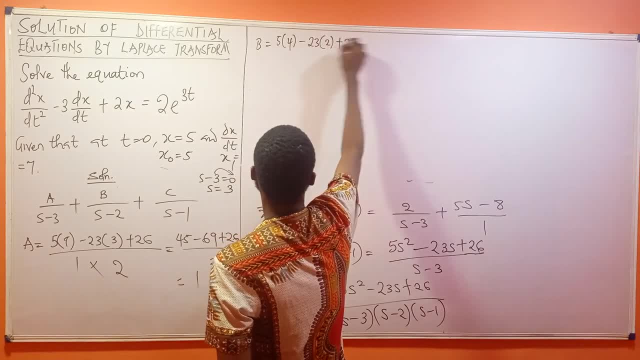 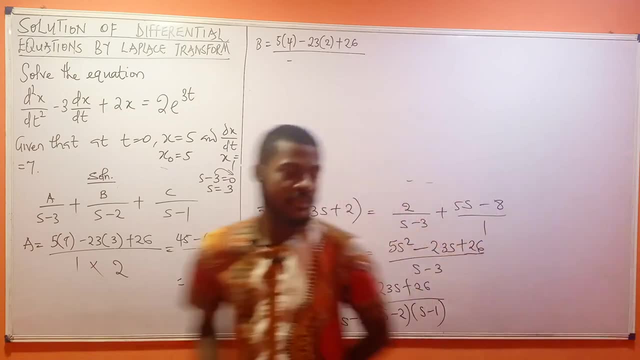 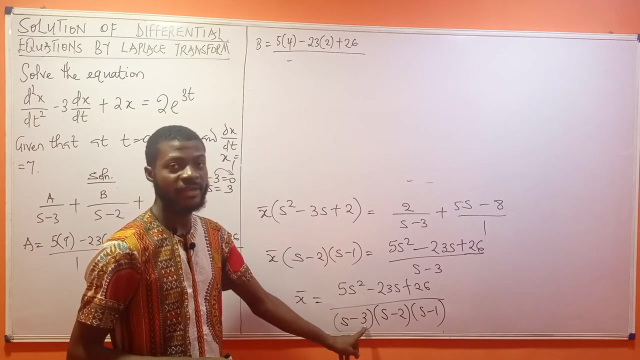 minus twenty three brackets. two plus twenty six, divided by two minus three. Now denominator here says s minus three. This denominator says s minus three, And remember we're saying s should be two, So this is now two minus three. All I give to you minus one, So this is minus one times. 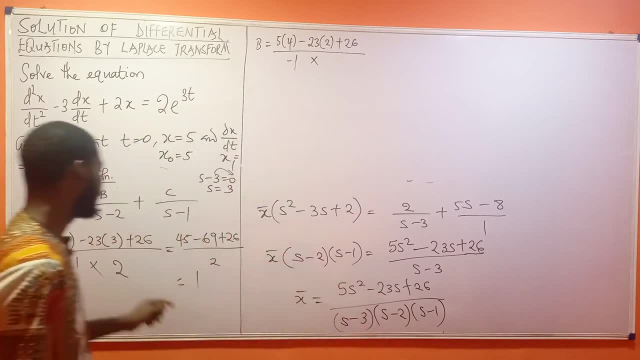 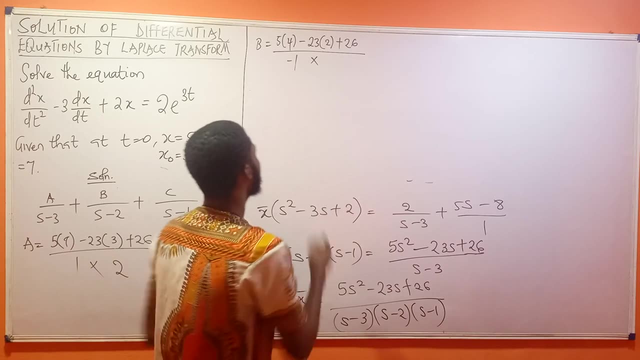 This s minus four I'm not going to be using. Remember why? Because that was the value we used to find our b. So I'm not going to be using. So s minus one. If we put two here, Two minus one is what One, So this times one. Now how will this be? 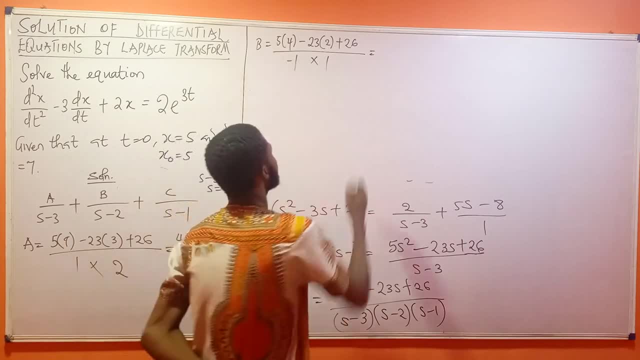 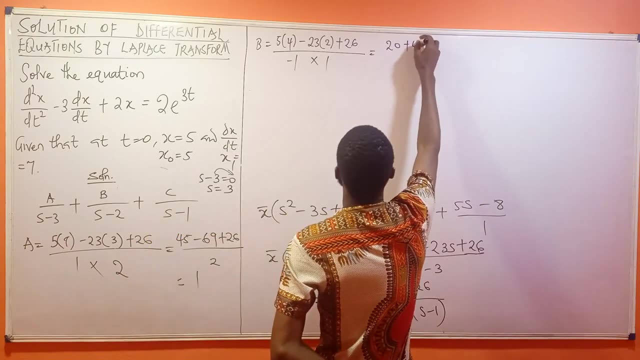 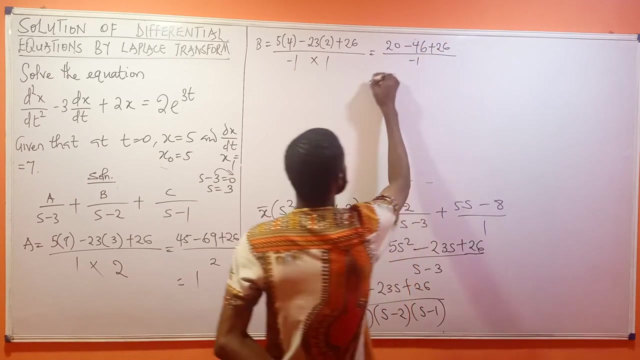 given to you Five times four will give you what? Twenty. So this is twenty. Then twenty three times two. What will that give to you? Forty six, Okay, sorry, Minus forty six. Then plus twenty six: All of our what Minus one. What will the answer of this be? 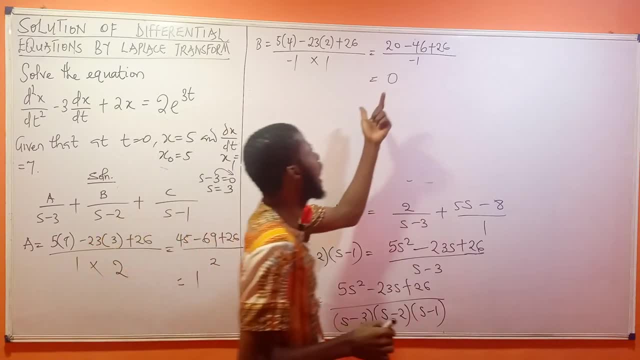 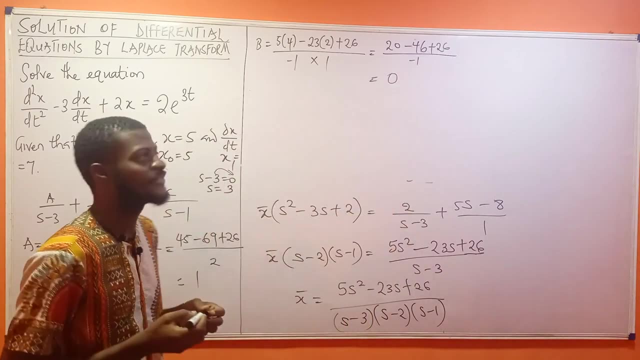 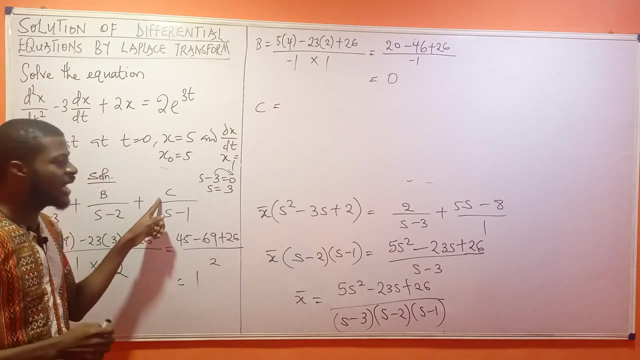 Zero. That's going to give you zero, Because twenty plus twenty six is forty six. Forty six minus forty six, That will give you zero. So this answer is kind of sweet. So your c? C will then become the last guy that we're going to be finding Now at the bottom of c, At the bottom of c, S minus one. 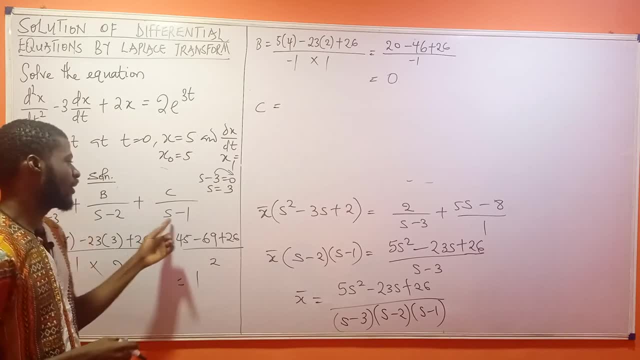 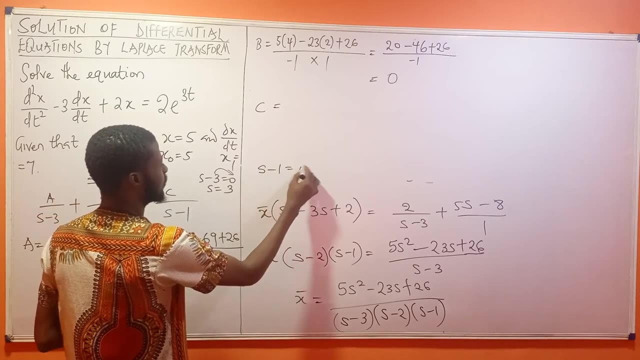 is what we have. Now I think let me just calm down. S minus one is what we have. So this s minus one guy, If you say s minus one Is equal to zero, What will be your s? finally, This minus one will go over. So s is equal to what? 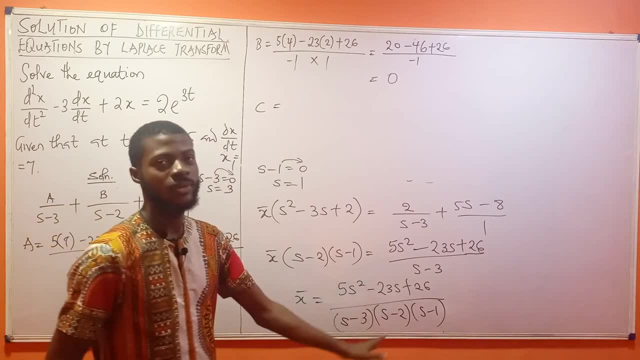 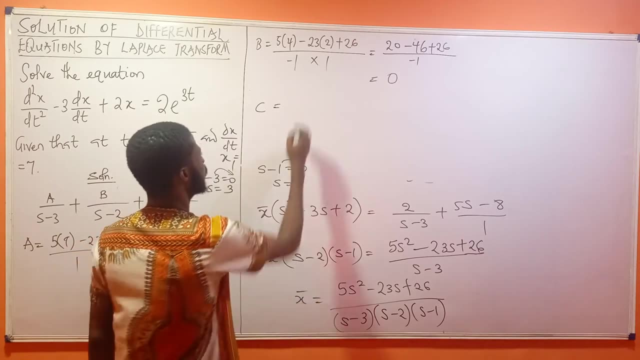 One. So anyway, you see, s You are going to be putting what One, That's the meaning, And I think it's very easy if we're dealing with one, So we are just using the numbers in front of it. So this: 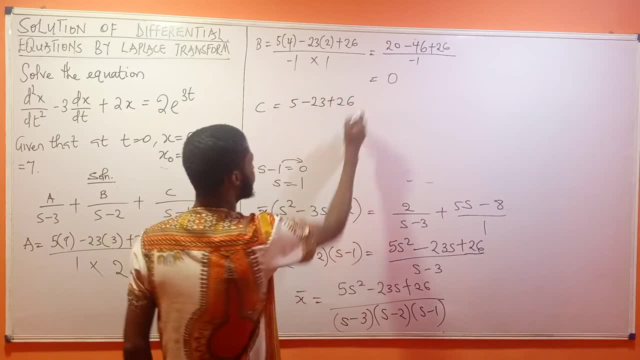 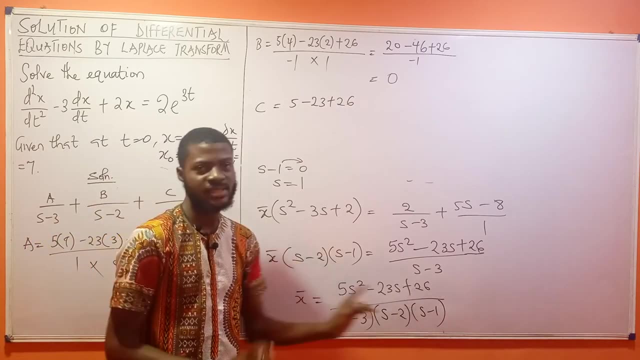 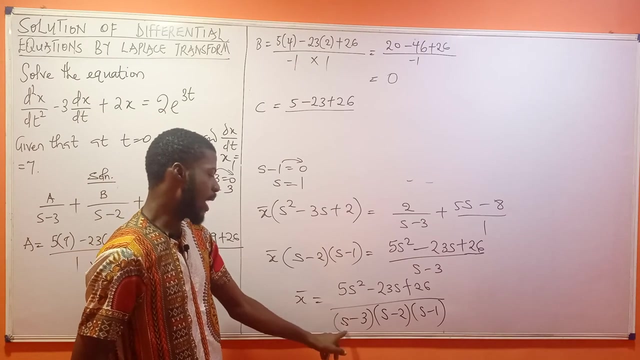 just become five minus twenty, three plus twenty six. You know why. One times anything is that same thing. So that's why I just use five minus twenty, three plus twenty six. It's easy that way. Denominator, If you are putting one, Don't make that mistake. please Put one here, One minus three. 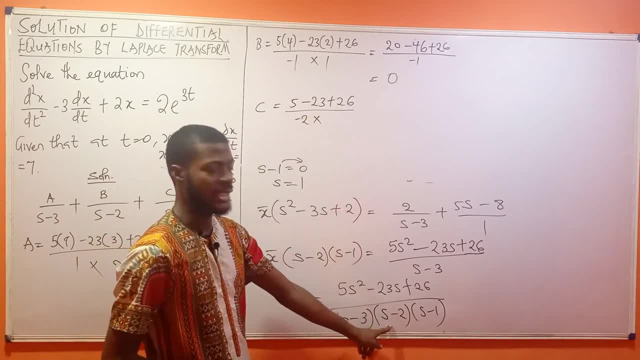 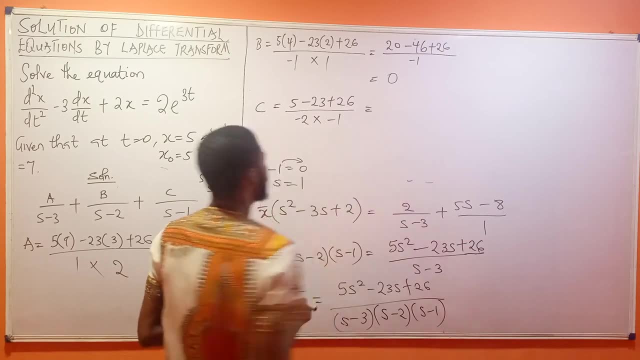 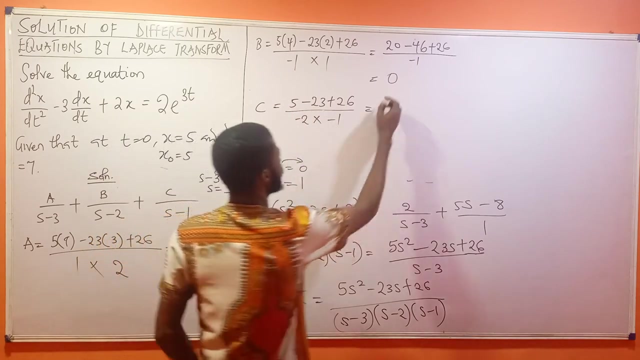 is minus two. Then times Put one here: One minus two is what Minus one. Remember you won't be using the x minus one, So this will not be equal to Twenty. six minus twenty. three will give you what Three. Three plus five is what Eight. So this is eight over two, which is what Four. So I've 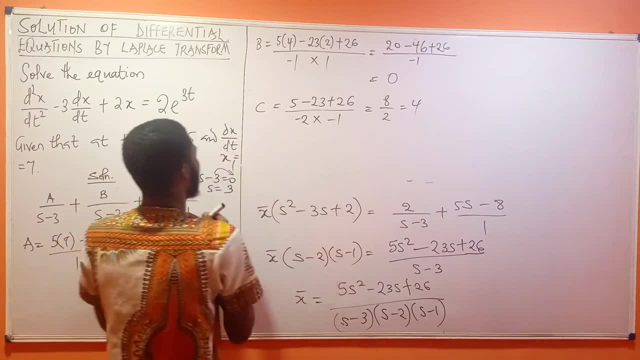 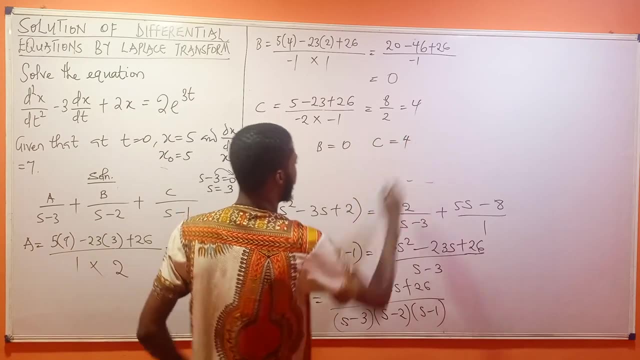 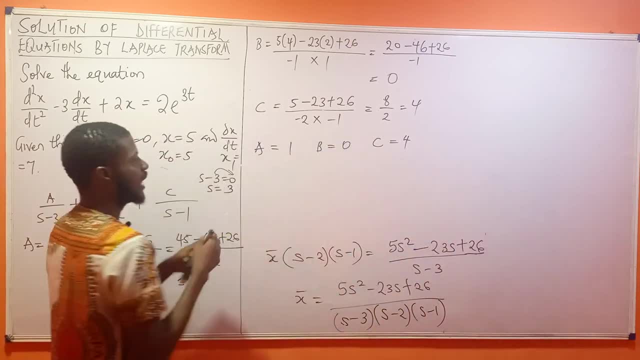 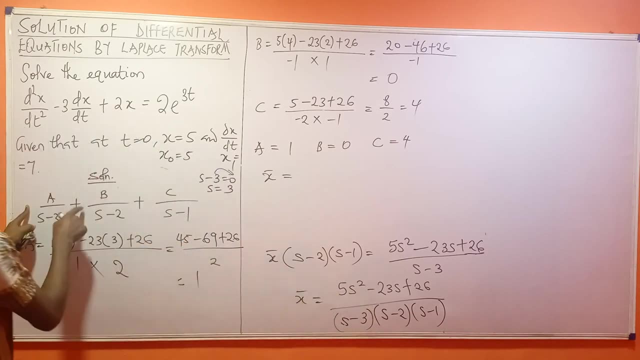 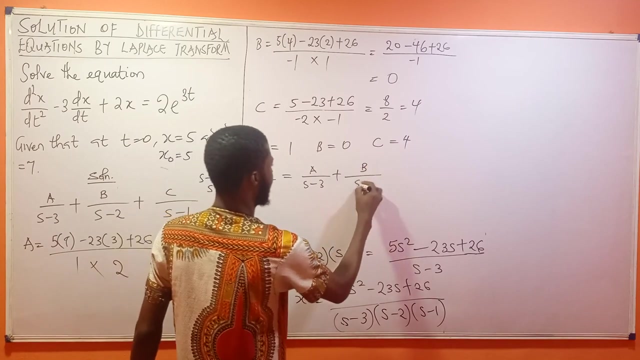 Now remember. Remember that we said s bar is equal to this fraction that we have here, Because this is what we're trying to solve. So we said it's equal to this. So our s bar is equal to a over s minus three plus b over s minus two plus c. 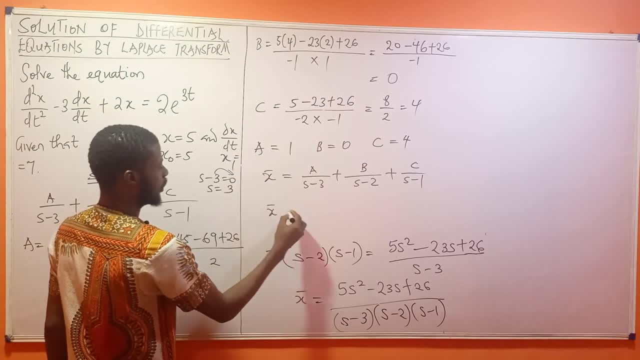 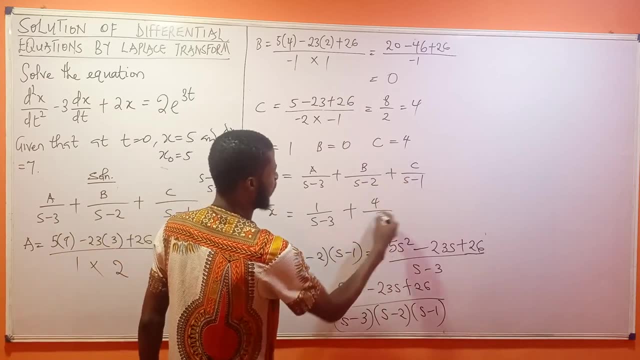 over s minus one, So this is s bar equal. What is a: a is one, So this is one over s minus three plus What is c? Four over s minus one. I didn't talk about the b, because if I put zero here, 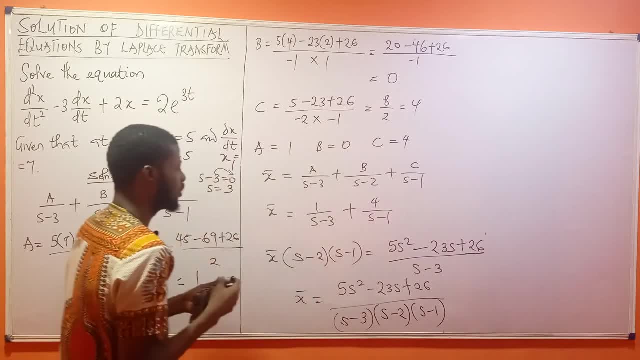 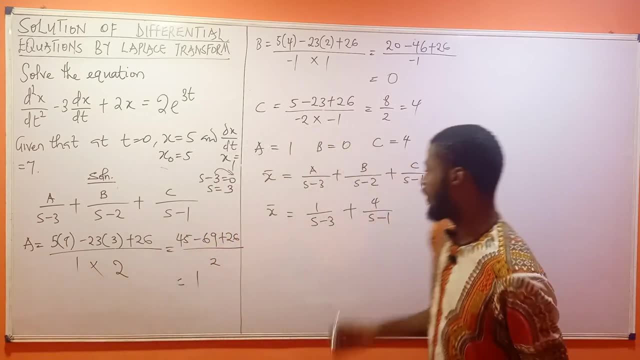 zero over anything is zero, So that's quite useless. So this is the expression that we now have. So this is the resulting expression that we have Now. for this very expression, we've done everything we can do. The last thing to do is to do the problem piece. 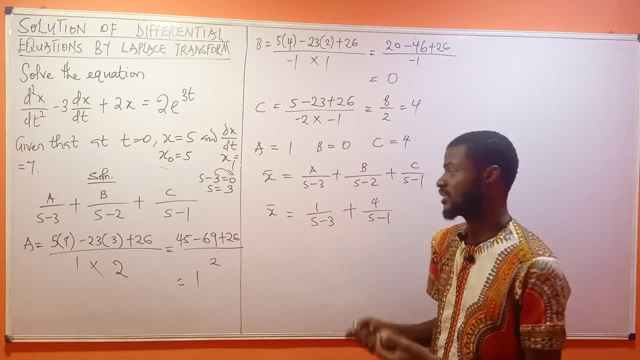 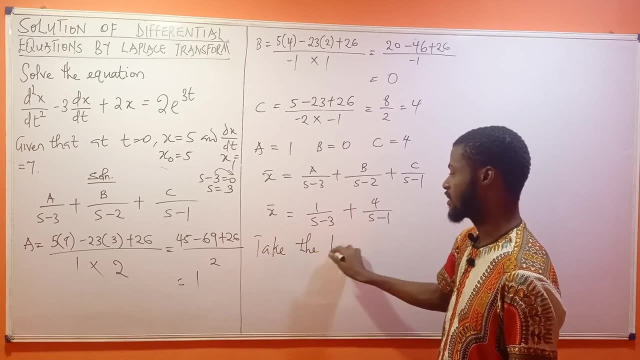 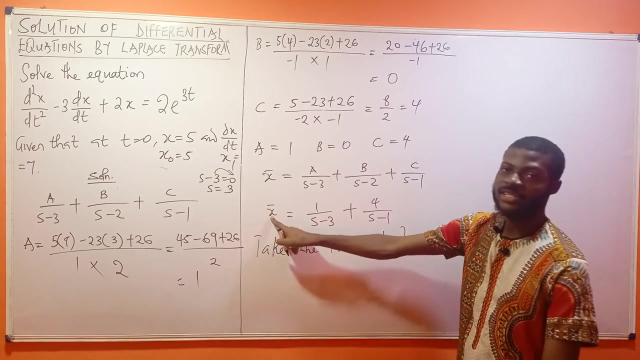 do is to what find the what inverse laplace, transform of everything that we have here. so what's the inverse? let me just write it: take the inverse laplace, take the inverse laplace of everything that we have here. so what's the inverse laplace of s bar? 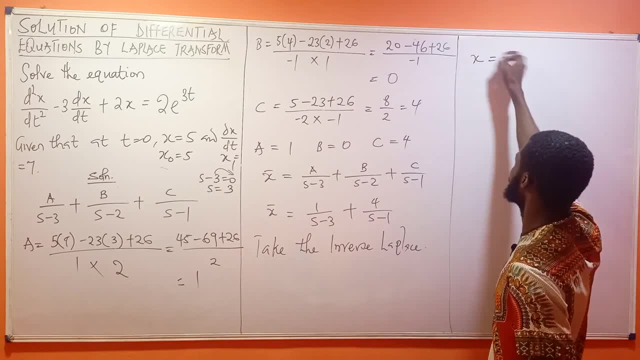 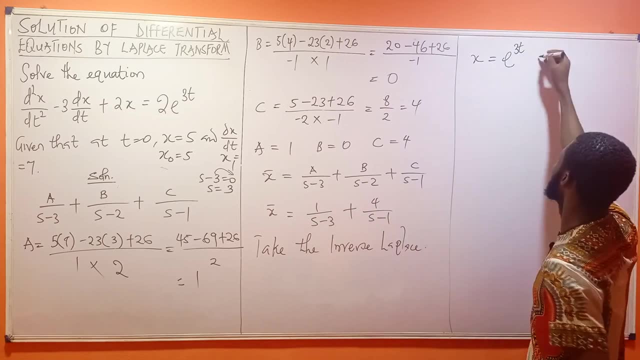 that will give you x. so this is s equal. what is the inverse laplace of this very guy? you're going to have e to the power of three t, then um plus, what are you going to be having? you're going to be having four e to the power of c. so that is what, the final answer to this very question.